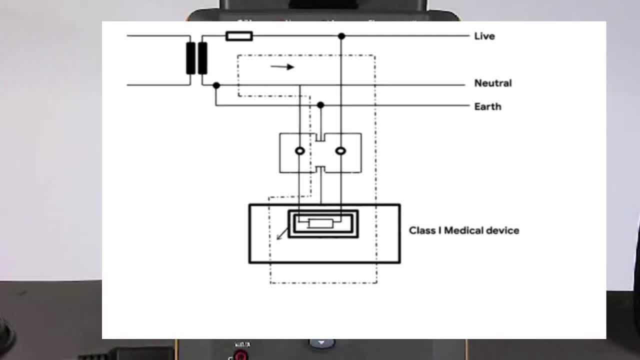 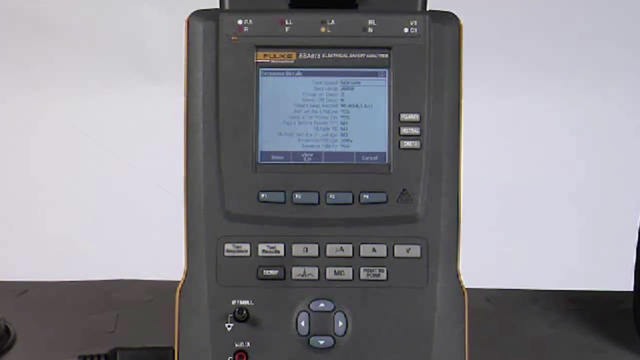 A large fault. current flows from the mains part to earth via the protective earth conductor, which causes a protective device, usually a fuse in the main circuit, to disconnect the equipment from the supply. It is important to realize that not all equipment having an earth connection is necessarily Class 1.. 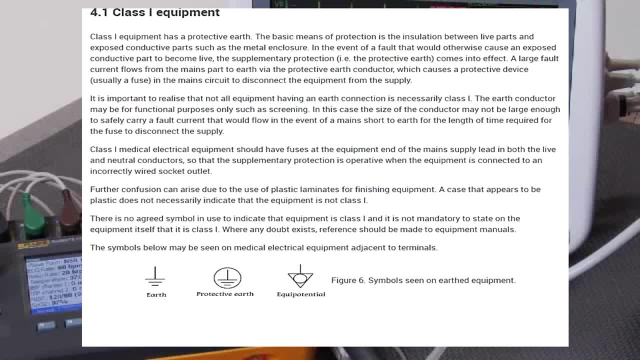 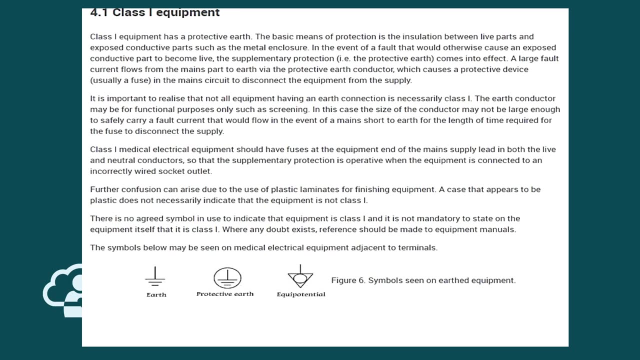 The earth conductor may be for functional purposes only, such as screening. In this case, the size of the conductor may not be large enough to safely carry a fault current that would flow in the event of a main short to earth for the length of time required for the fuse to disconnect the supply. 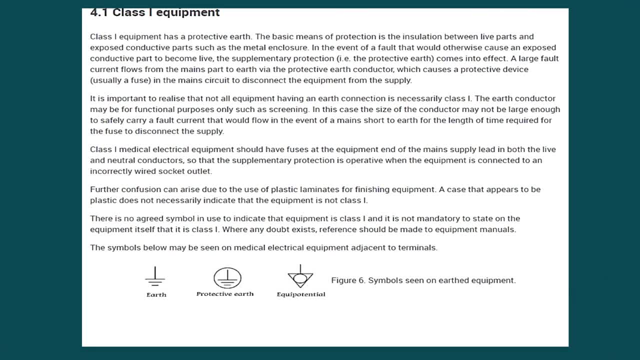 Further confusion can arise due to the use of plastic laminates for finishing equipment. A case that appears to be plastic does not necessarily indicate that the equipment is not Class 1.. There is no agreed symbol in use to indicate that the equipment is Class 1,. 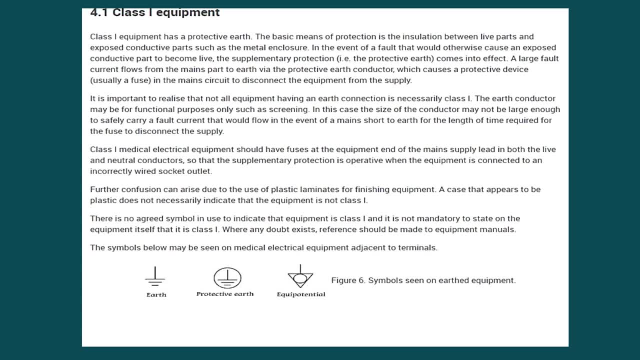 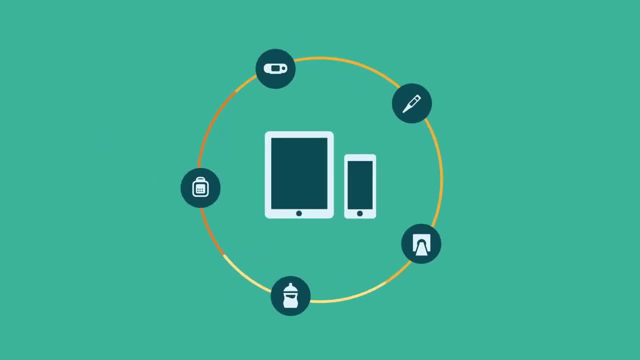 and it is not mandatory to state on the equipment itself that it is Class 1.. Where any doubt exists, reference should be made to equipment manuals. Let's move towards Class 2 equipment. The method of protection against electric shock in the case of Class 2 equipment is either double insulation. 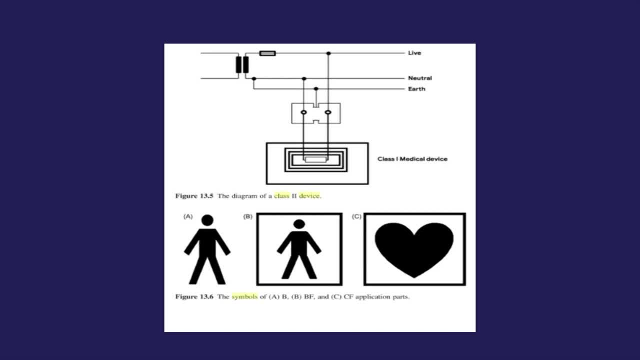 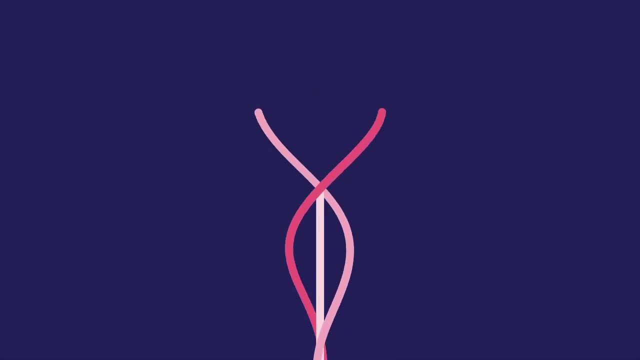 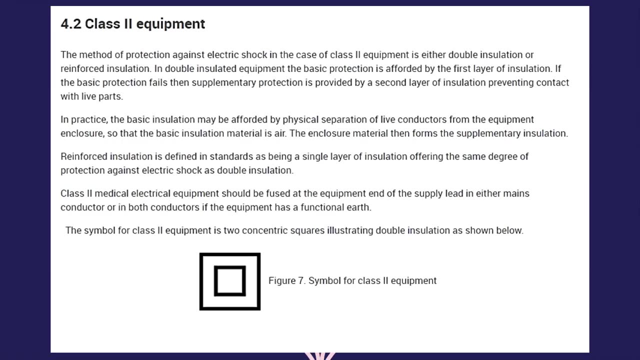 or reinforced insulation. In double insulated equipment, the basic protection is afforded by the first layer of insulation. If the basic protection fails, then supplementary protection is provided by a second layer of insulation preventing contact with live parts. In practice, the basic insulation may be afforded by physical separation of live conductors from the equipment enclosure. 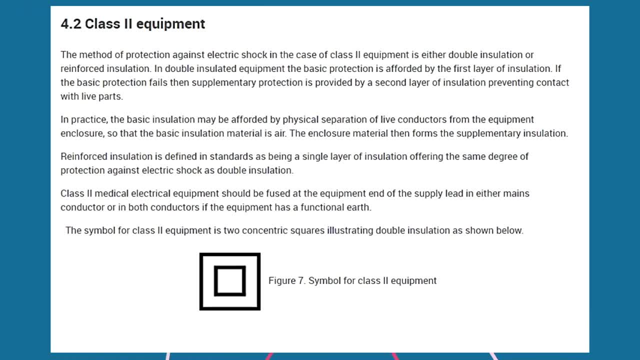 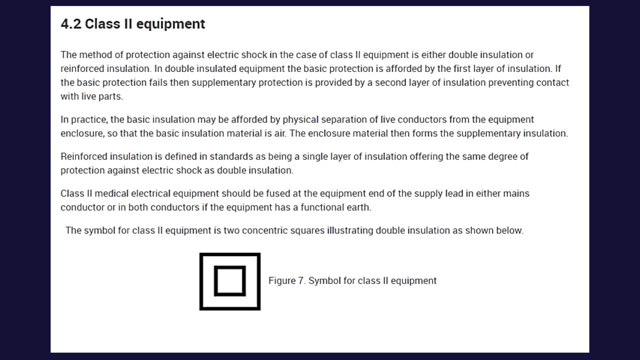 So that the basic insulation material is air. The enclosure material then forms the supplementary insulation. Reinforced insulation is defined in standards as being a single layer of insulation offering the same degree of protection against electric shock as double insulation. Class 2 medical electrical equipment should be fused at the equipment end of the supply lead.